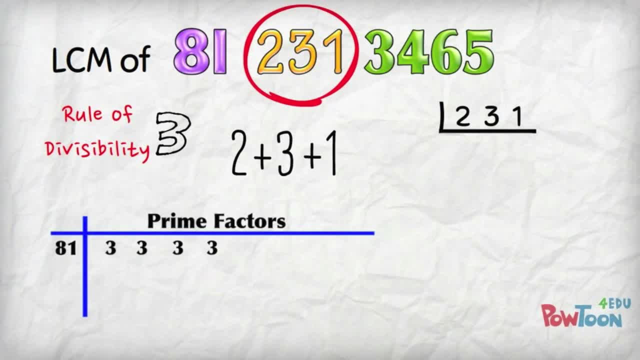 When I add these digits, 2 plus 3 plus 1, I get 6.. So I know 3 is a factor 231 divided by 3, 3 x 23, 7 x 3 is 21, Remainder 2. 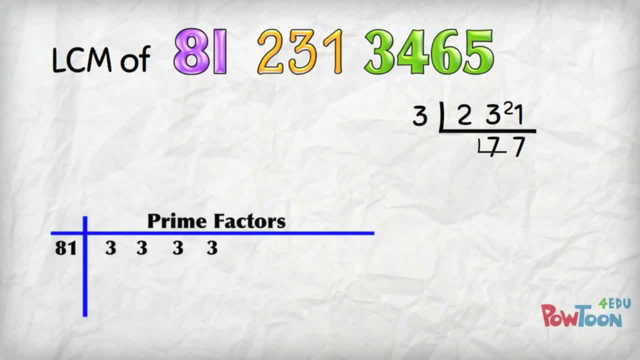 3 x 21. 7 x 3 is 21, 77. I'll divide by 7. 11 x 7 is 77. 11 is prime. 11 x 11. 1 Write in the prime factors of 3. 231. 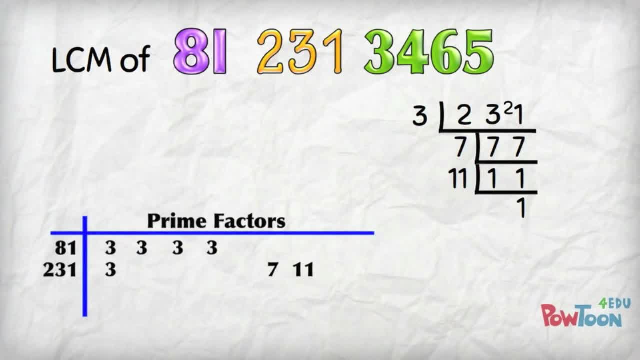 3 x 7 x 11. And now for the big one: 3465. Obviously, this calls for the Short Division to extract the primes. Our number ends in 5, so we can instantly tell that 5 is a factor. So start off by dividing by 5.. 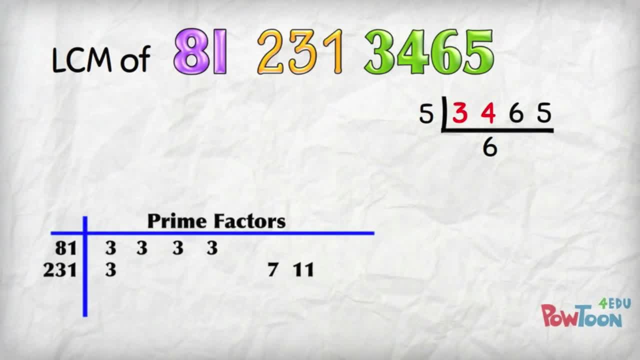 5 x 34. 6 x 5 is 30. Remainder 4, 5 x 46. 9 x 5 is 45. Remainder 1, 5 x 15, 7 x 15. 3 x 5 is 15. 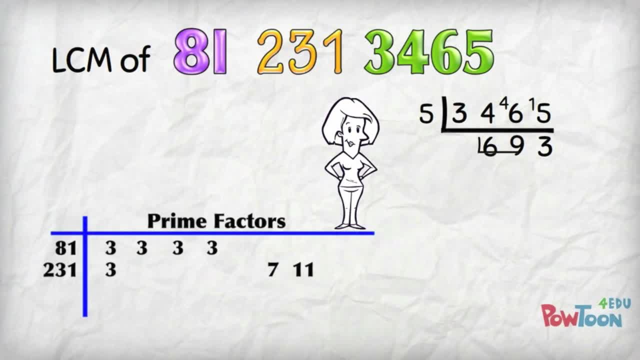 693, I can tell immediately that this is divisible by 3, because each individual digit is divisible by 3.. No need to add the digits this time, Just apply your common sense. 3 x 6, 2 x 3 is 6. 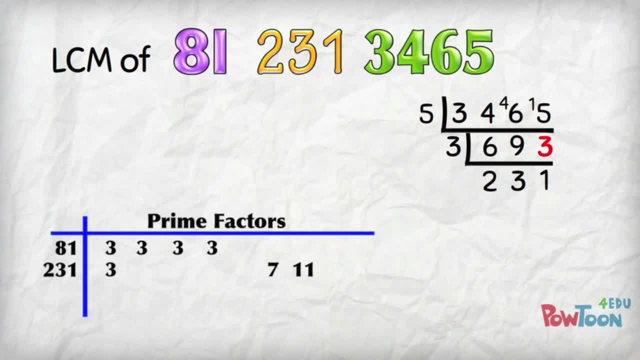 3 x 9. 3 x 3 is 9, 3 x 3 is 1: 231. What a coincidence. We've just done 231!. We know its factors already. Let's save some time I can write in the prime factors that I found through Short Division so far. 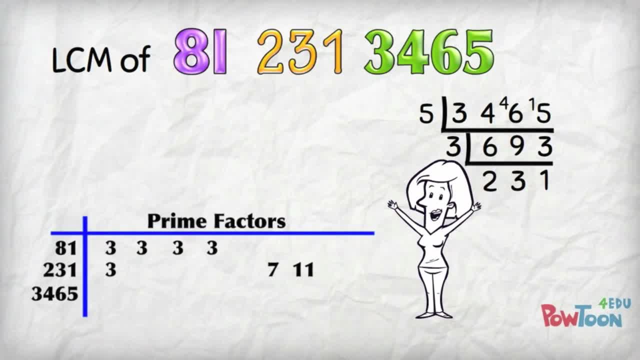 then repeat the factors of 231.. It isn't cheating, since I did the work once already. So we've got 3 x 5 and then, from 231, 3 x 7 x 11. So the factors of our mystery LCM are: 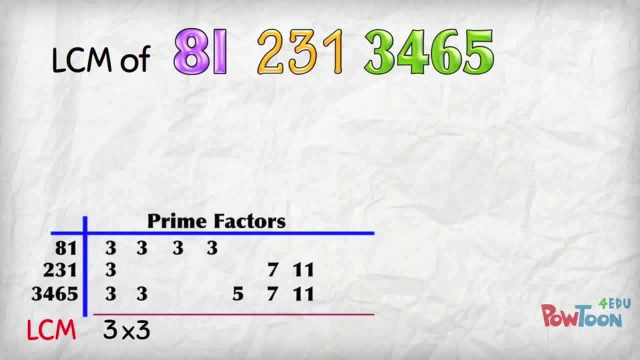